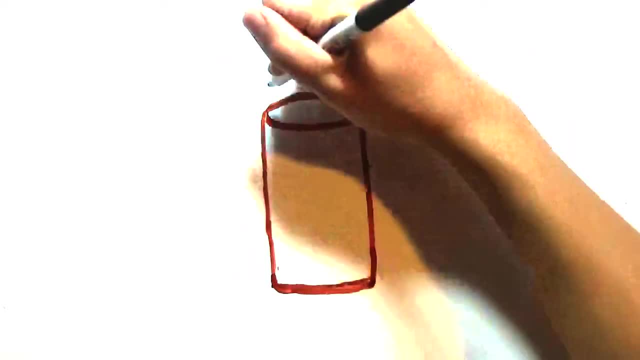 nuclear waste can still be stored in casks for a hundred years, and even if it is stored for a hundred years. it can still be stored for a hundred years, and even if it is stored for a hundred years or more, before requiring maintenance. some prefer to bury waste for. 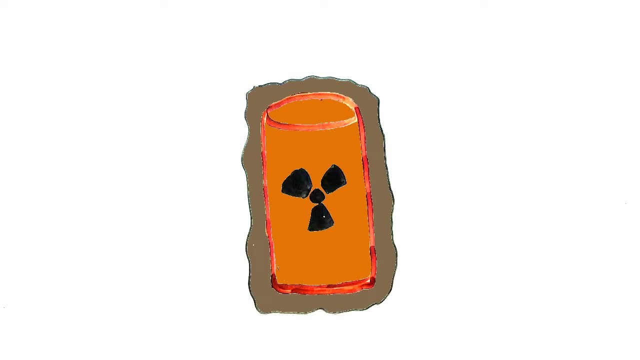 longer periods in ground storage. This can be done through placing the nuclear waste within non-corrosive copper structures, surrounding them with clay which protects the seal of the copper structures, then placing the vessel 500 meters below ground surface in hard crystalline. 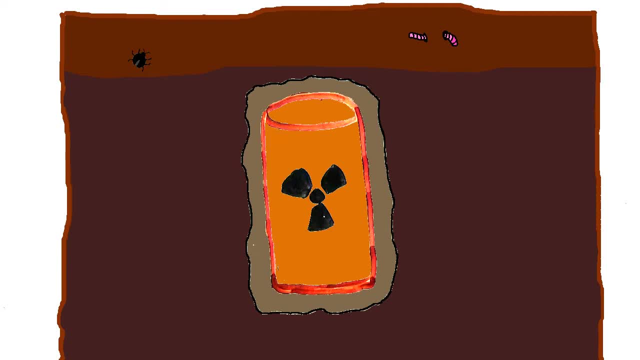 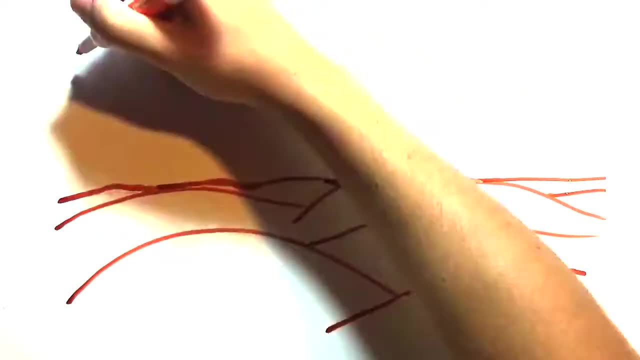 bedrock, though there is still some potential contamination with groundwater. Other nuclear repositories, however, like one which was planned for the Yucca Mountain Wastelands of Nevada, store nuclear waste above the water table in underground packages. There are even deep. 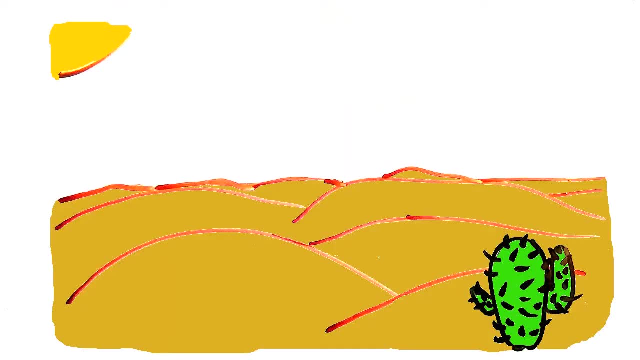 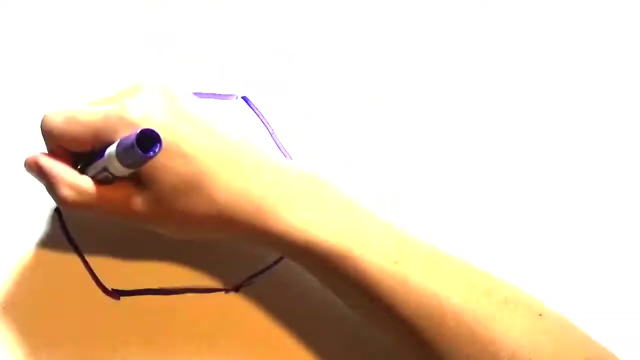 borehole. methods involving burying contaminated material 3 to 5 kilometers underground surface, where water is isolated, and glass encasing methods involving mixing the contaminated material into molten glass, which entraps radiation and hardly breaks down over time. Such methods cannot always be implemented, as in earthquake-prone Japan, where casks 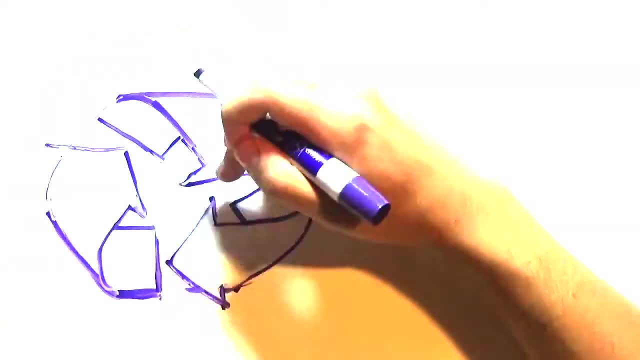 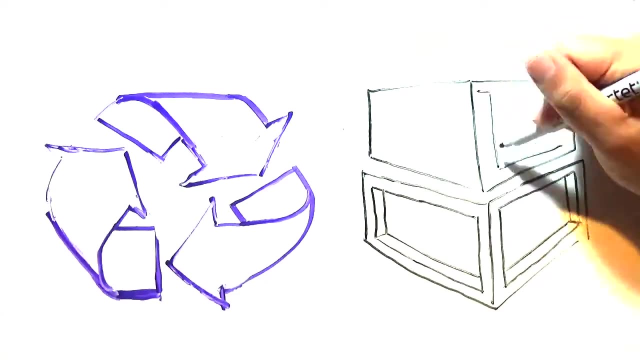 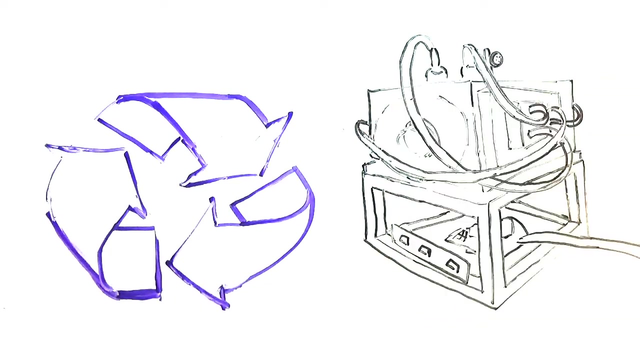 may be used, but underground storage cannot be. but the more expensive the material, the more expensive. measures of reprocessing and recycling are becoming popular globally. In South Korea, for example, a 500 degree Celsius veloxidizer oxidizes unstable uranium dioxide pellets into stable U3O8 powder, and in Russia, the revolving plasma within fusion reactors. 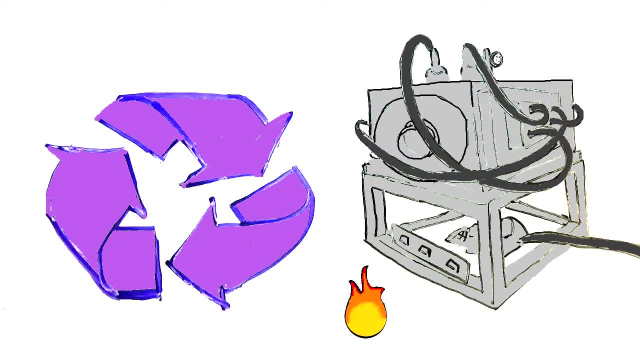 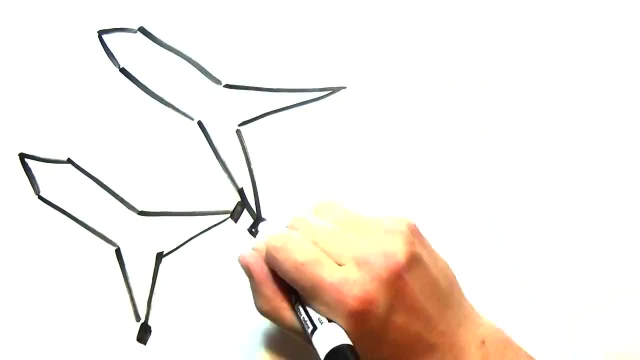 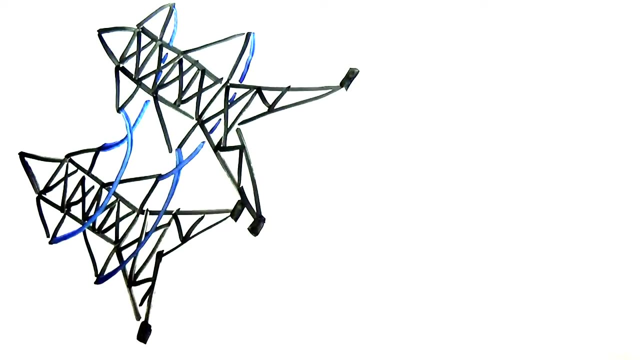 may be used as a centrifuge to separate components of radioactive waste from one another for effective reprocessing, among other separation techniques. The prospect of nuclear reactions in the way of diversifying a nation's renewable energy has encouraged hundreds to sprout up around the world, despite the possibility of stored nuclear waste being accessed by 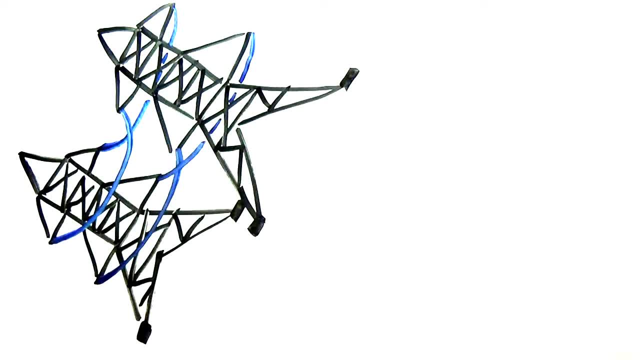 violent groups. Even so, alternatives like thermal solar power focus light energy from the sun's own nuclear reactions to generate steam and power turbines similar to how a nuclear reactor spins turbines with steam and are arguably more sustainable, as there is a limited supply of not only nuclear materials but also materials which are used during the 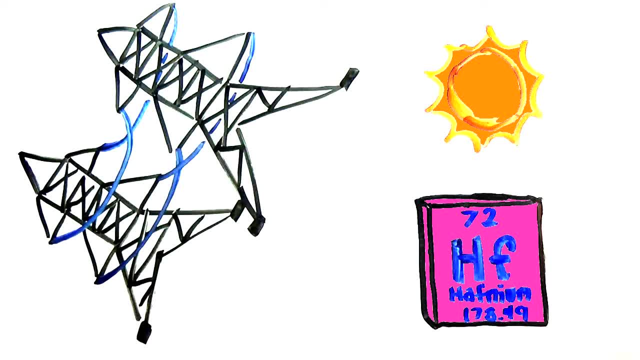 processes like nuclear power plants, nuclear power plants and nuclear power plants. The use of nuclear power plants and nuclear power plants in nuclear power plants is a key factor in the development of nuclear power, Like hafnium, a metal used to bring great integrity to superalloys.